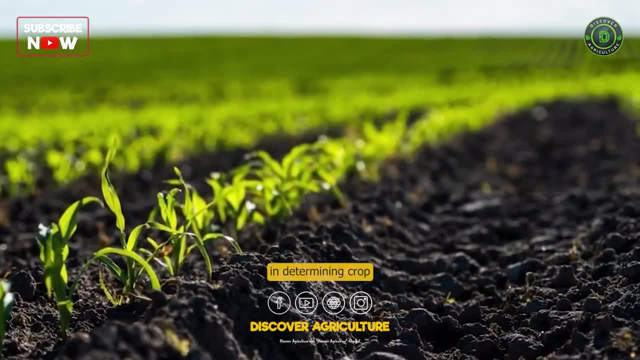 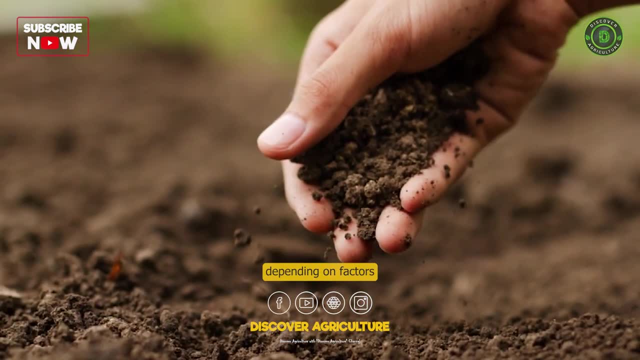 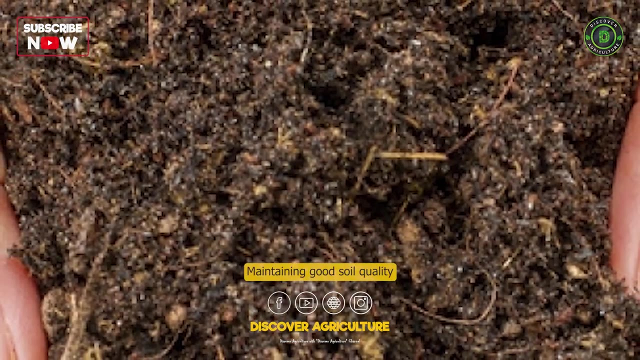 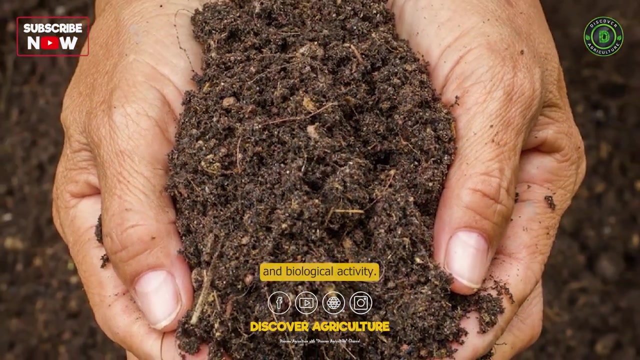 Soil quality on a farm is a critical factor in determining crop productivity and sustainability. The quality of soil can vary widely depending on factors such as soil type, previous land use and management practices. Maintaining good soil quality on a farm requires careful management of soil structure, nutrient levels and biological activity. 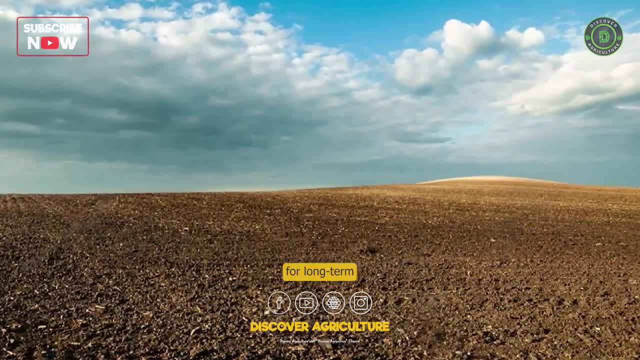 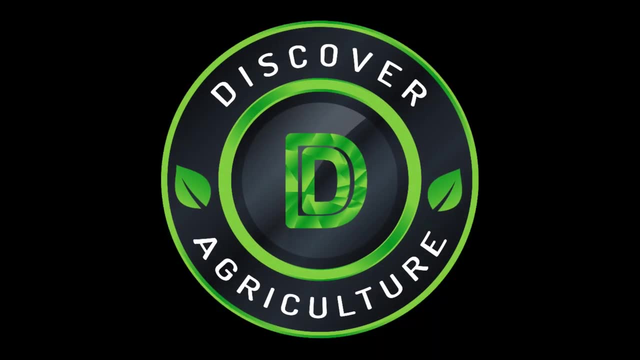 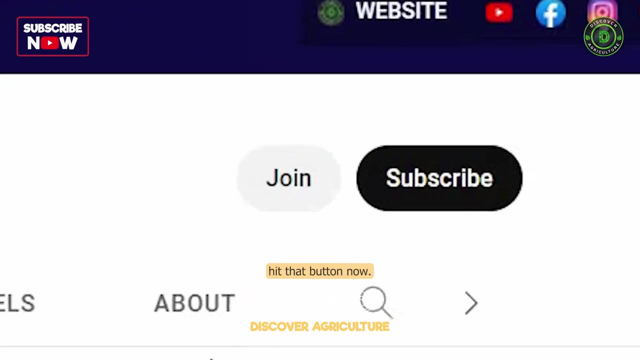 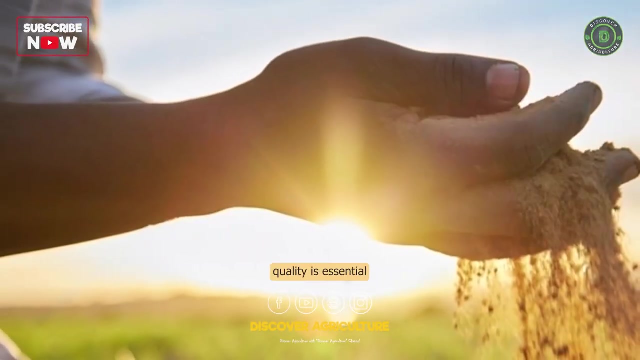 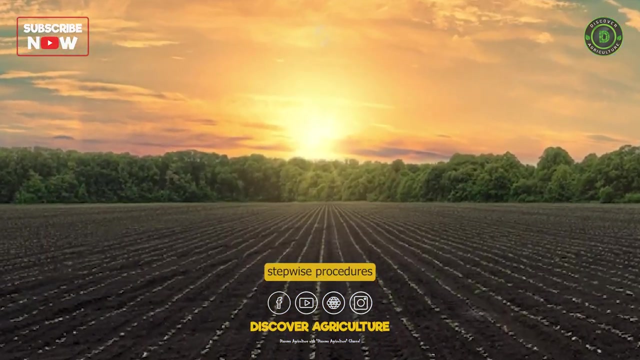 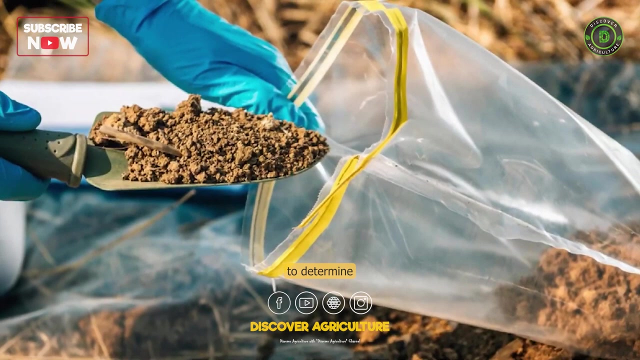 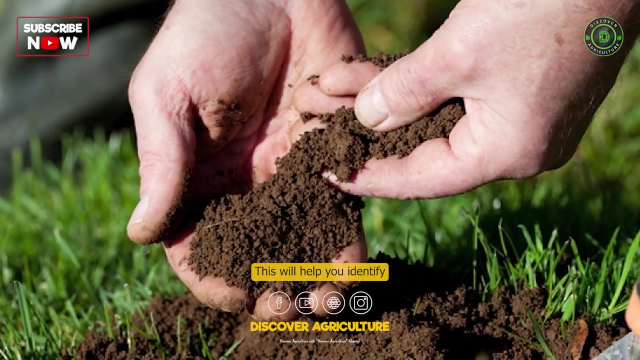 Investing in soil health is essential for long-term profitability and environmental sustainability in agriculture. Here are some stepwise procedures for improving soil quality on a farm: Soil testing: Start by testing your soil to determine its nutrient content, pH level and other characteristics. This will help you identify any deficiencies. 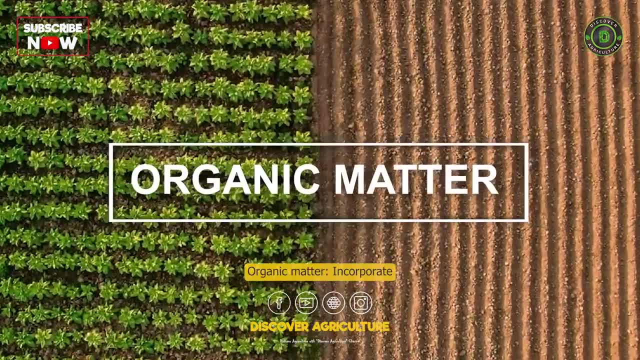 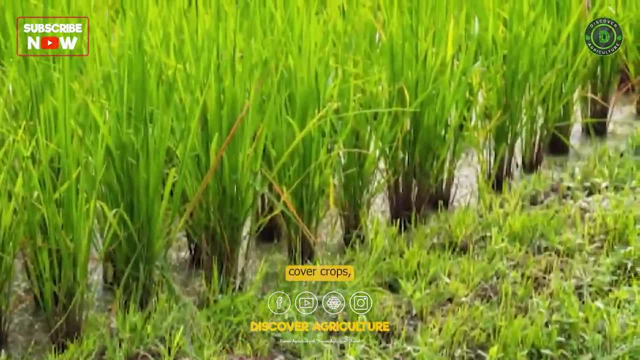 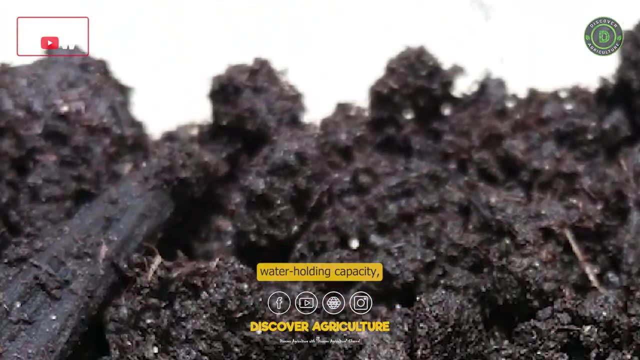 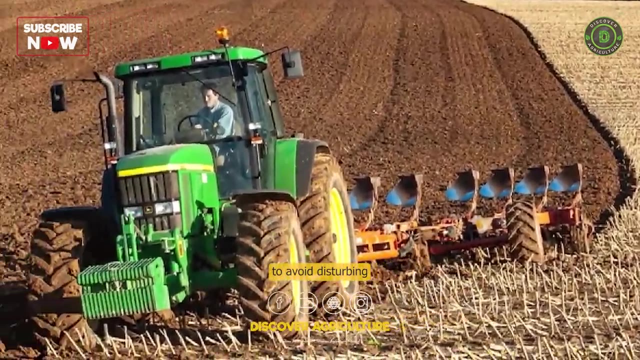 or imbalances that need to be corrected. Organic matter: Incorporate organic matter into the soil by adding compost, manure, cover crops or other organic material. Organic matter improves soil structure, water holding capacity and nutrient availability. Soil tillage: Reduce soil tillage to avoid disturbing the soil structure and promoting 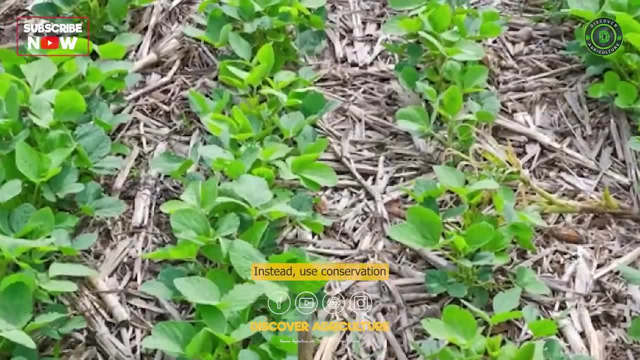 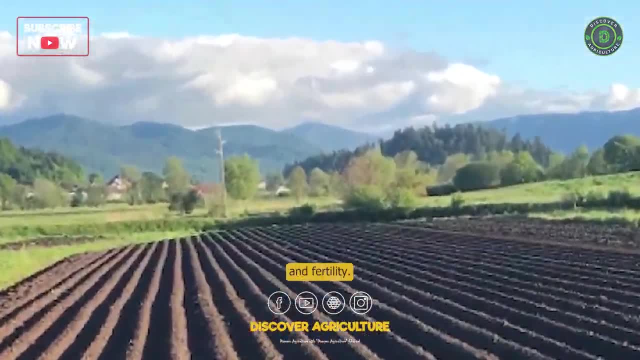 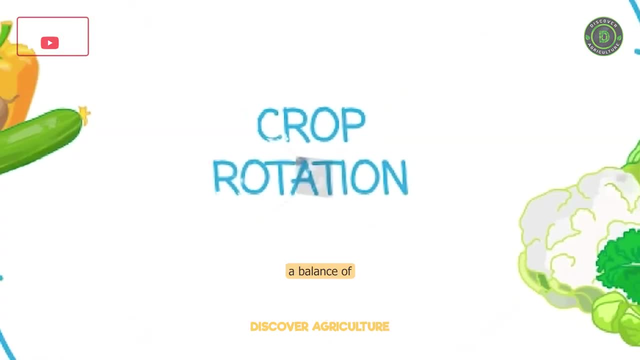 soil erosion. Instead, use conservation tillage practices such as no-till, reduce-till or strip-till to maintain soil health and fertility, Crop rotation, Rotate crops to prevent soil-borne diseases and pests and to maintain a balance of nutrients in the soil. 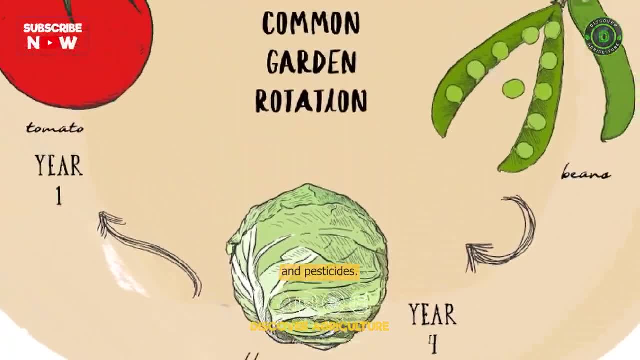 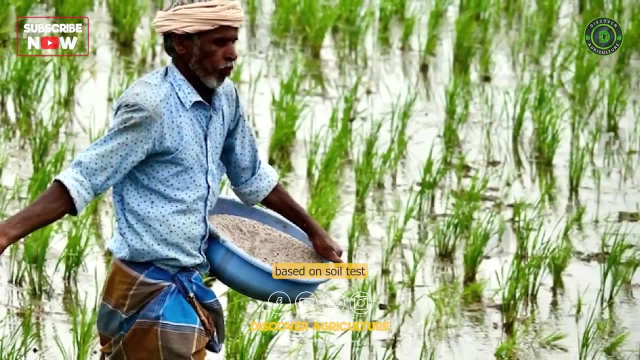 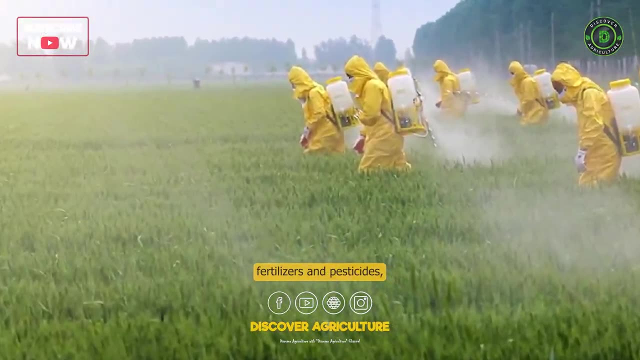 This helps to reduce the need for fertilizers and pesticides. Nutrient management: Use fertilizers and soil amendments wisely, based on soil test results and crop nutrient requirements. Avoid overuse of synthetic fertilizers and pesticides, which can harm beneficial soil organisms and lead to soil degradation. 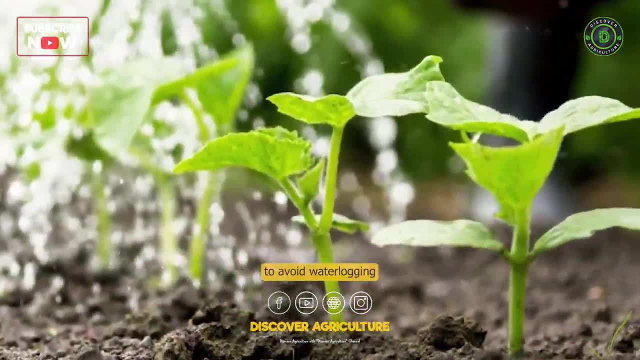 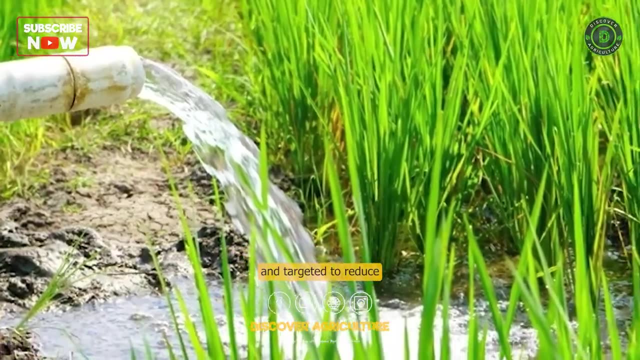 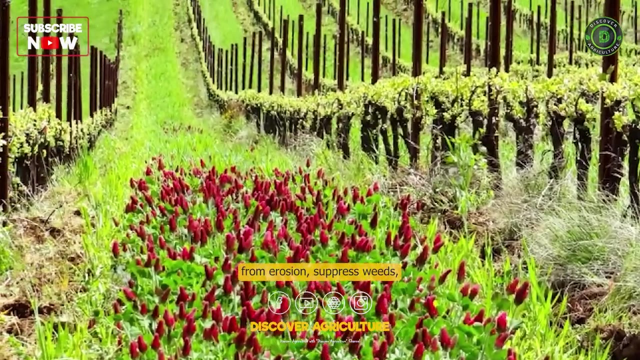 Water management: Manage water use carefully to avoid waterlogging or drought stress. Implement irrigation systems that are efficient and targeted to reduce water waste. Cover crops: Use cover crops to protect the soil from erosion, suppress weeds and add organic matter to the soil.